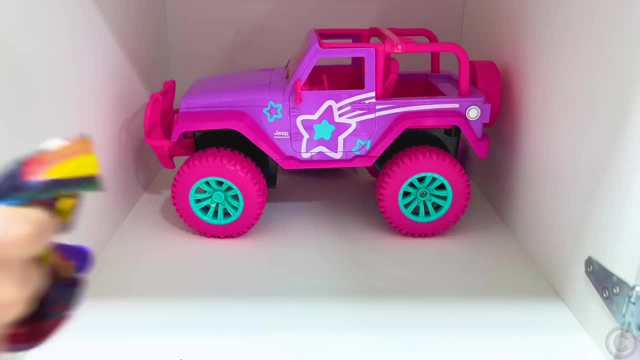 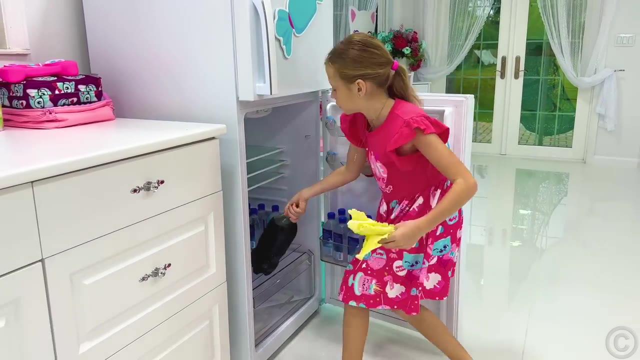 I'm ready to go. I'm ready to go. You're going to the park, Yes, Okay, One, two, three go. Okay, You're going to the park. Yeah, Okay, Okay, I'm going to the park. 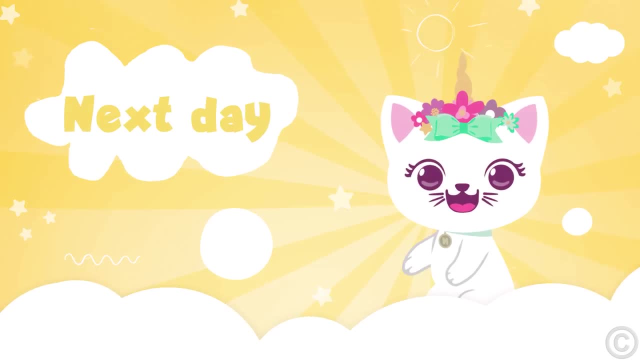 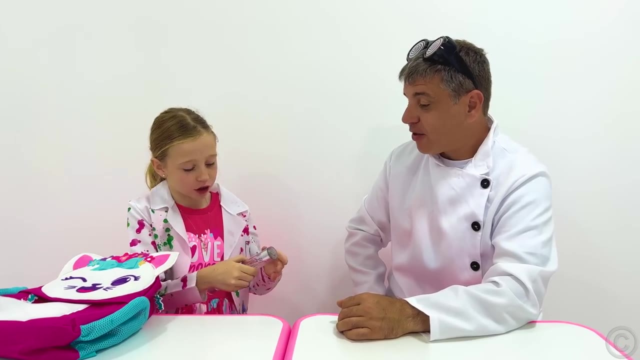 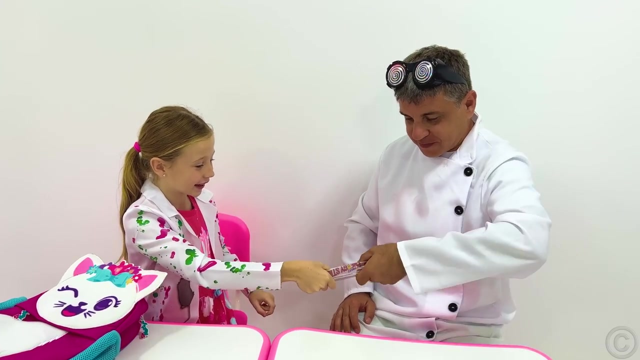 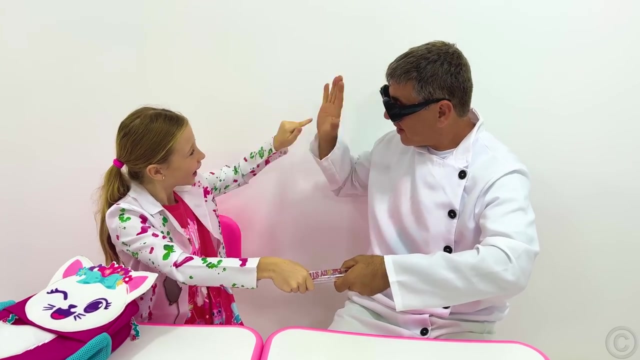 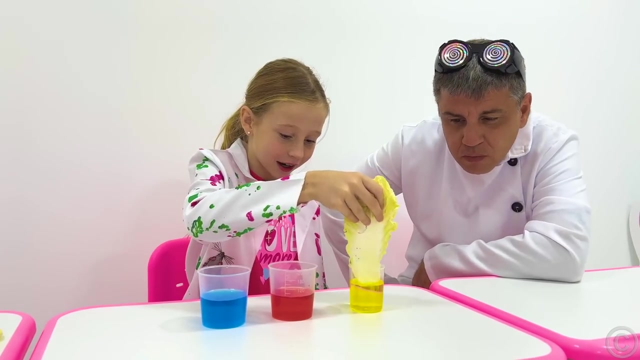 Okay, You're going to the park. Yes, Okay, You're going to the park. I'm going to the park, All right, the first one is an energy stick- look Cool. The second one is colored. We have to wait. 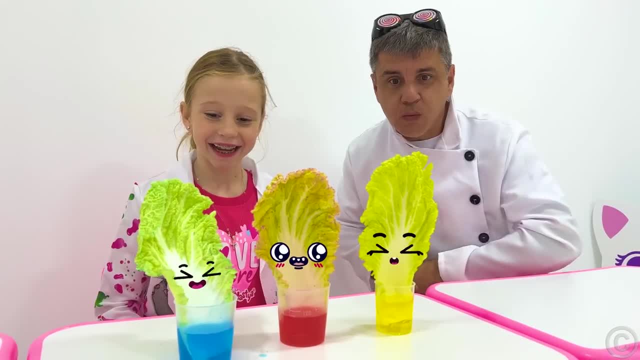 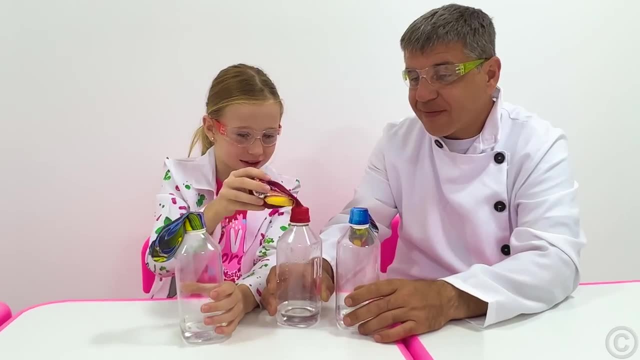 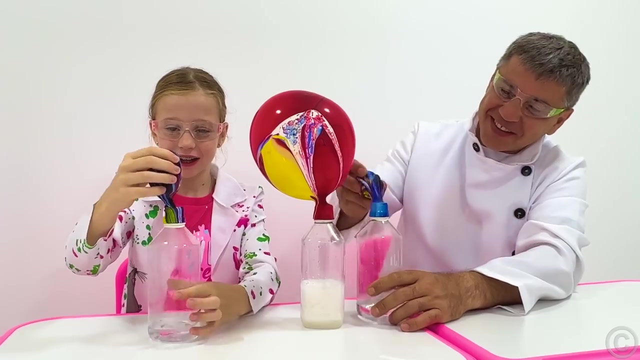 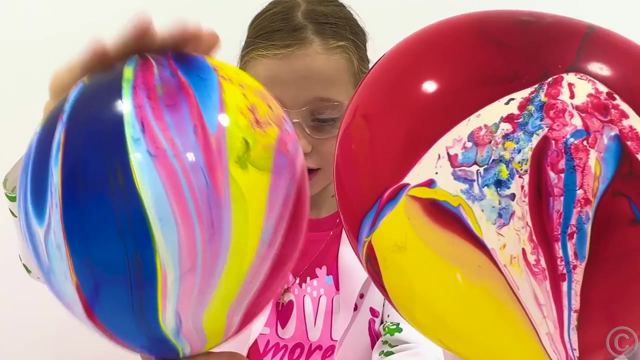 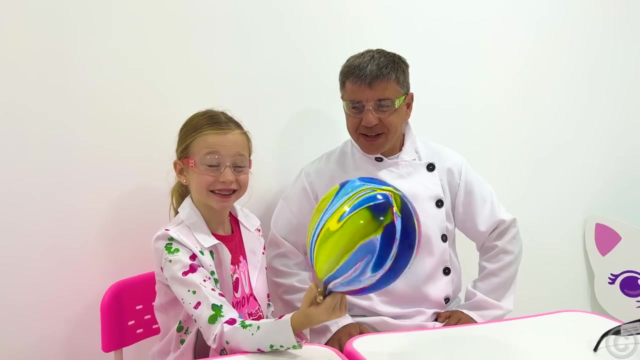 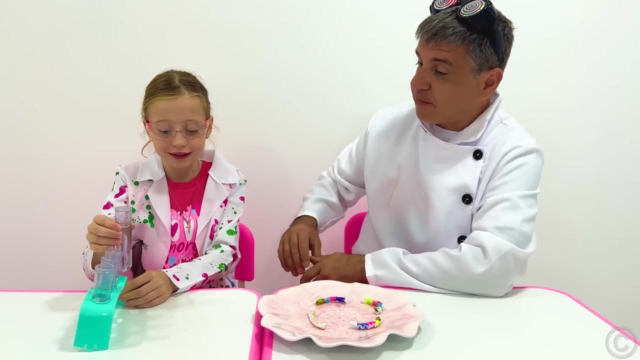 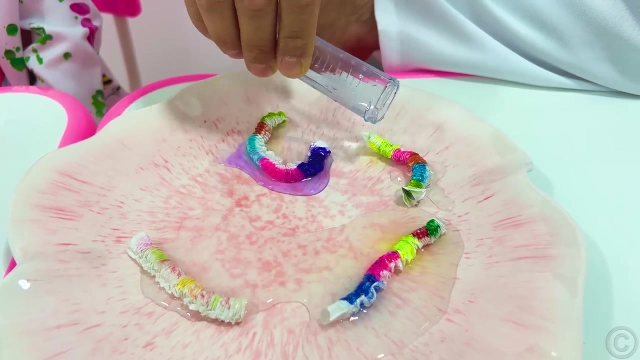 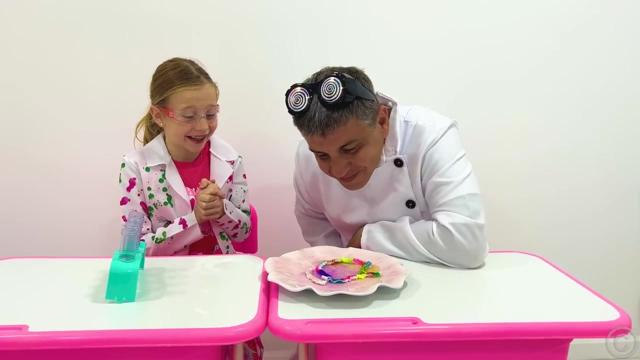 Okay, Ready, Let's blow balloons. Did you like it? Yeah, Paper worms, add some water, please. Okay, Ah, Are you ready? Are you ready for the crazy experiment? Yeah, Let's go up now, Oh. 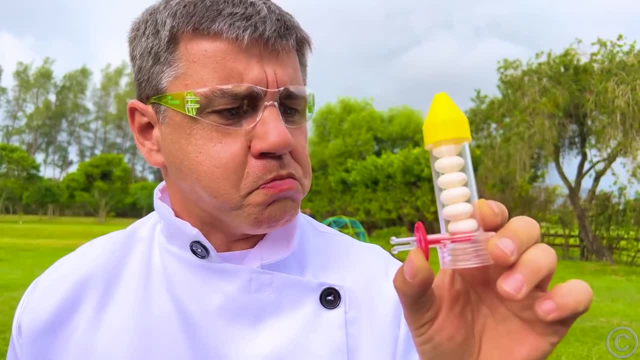 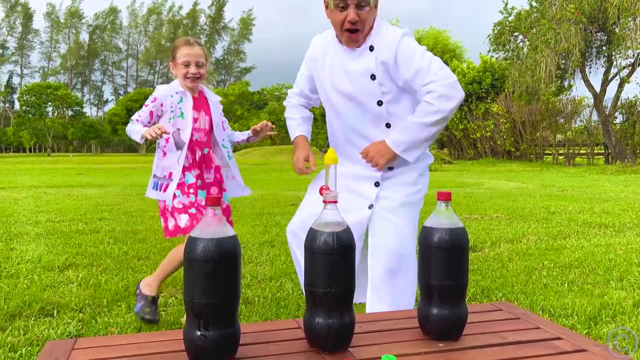 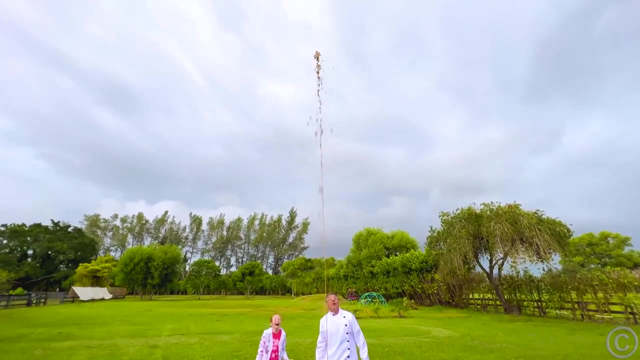 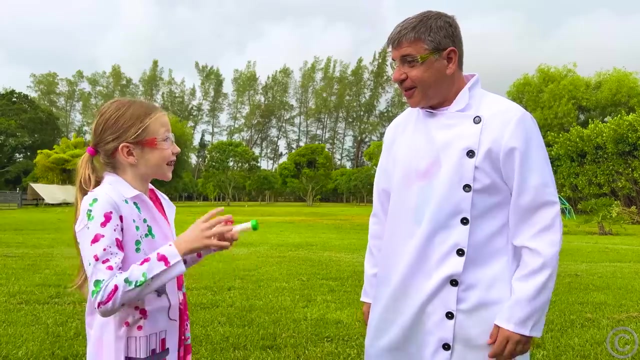 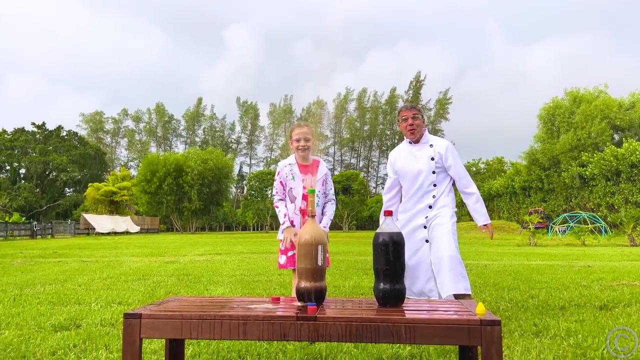 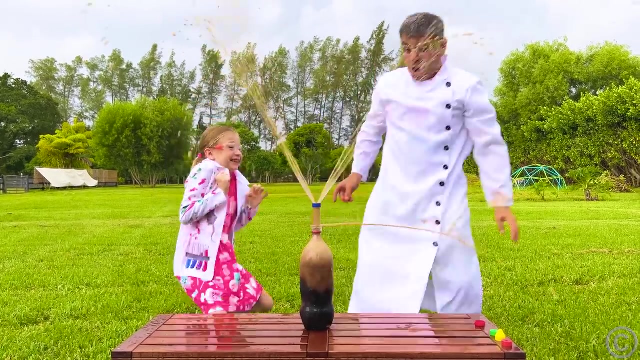 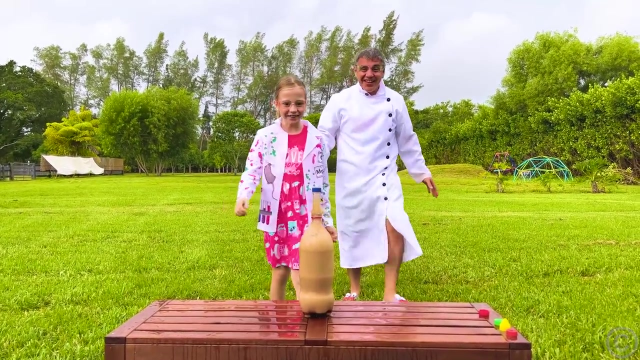 Add this in the bottle. Hmm, One, two, three, Three, Ah, Woo, Ah, Wow, Woo. Yay, The second one. Okay, Ah, I like science. Bye-bye guys, Bye.